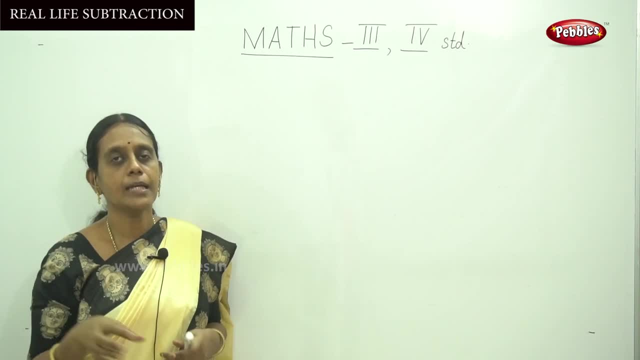 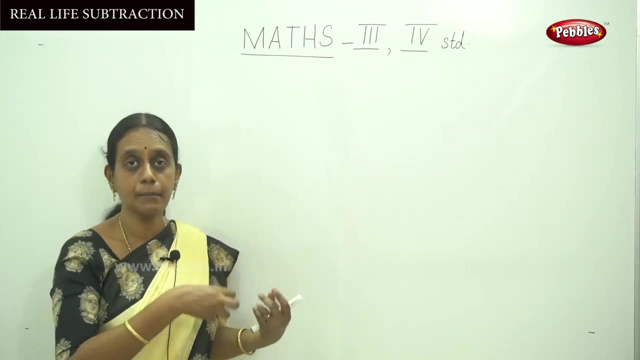 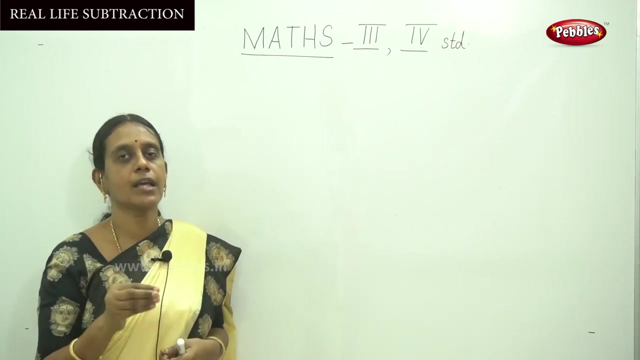 for a few things to purchase and come back to your home. Okay, That is, you have to calculate the difference amount, That is, the remaining amount in your hand. Okay, So that is the usage of subraction in real life. Okay, Let me see with example. 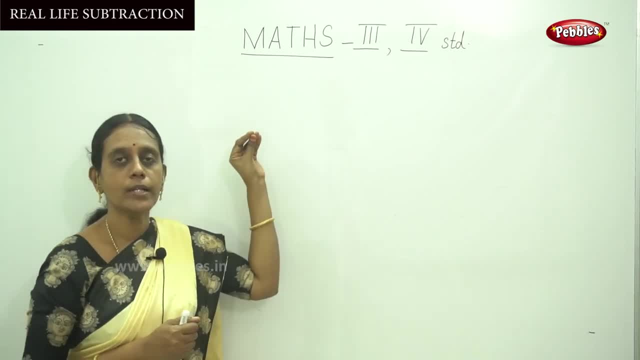 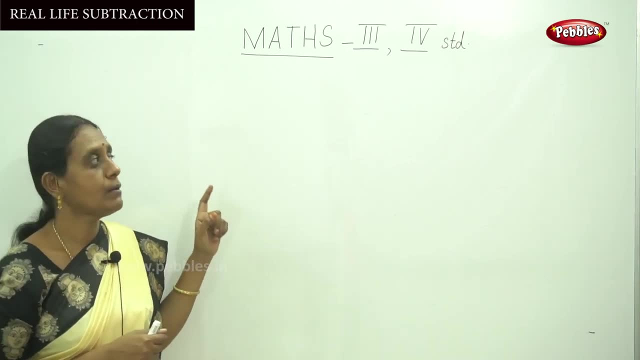 I will explain that is I am. I am going to write one word problem and explain the real life application That is. subraction is how much used in our day to day life. Okay, That is, let me do this. So that is how you calculate. Now let me tell you about the following. So 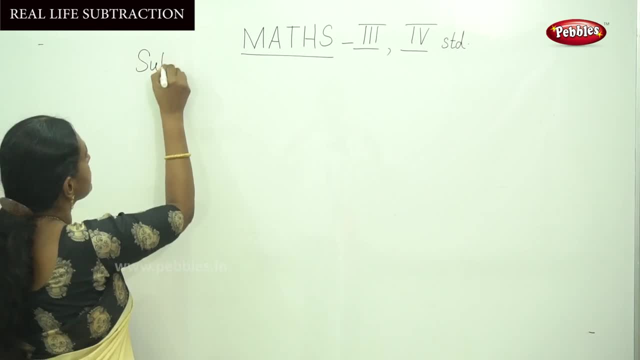 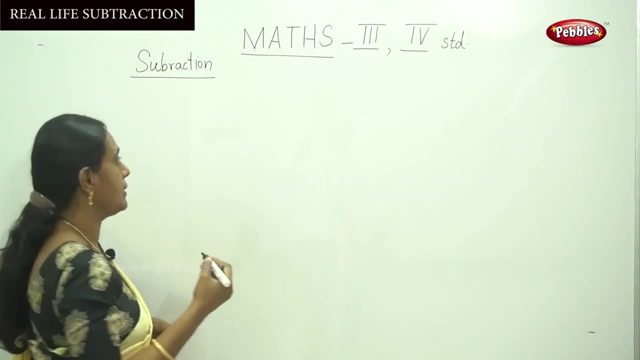 first point is that I am the subject. of course, I am not writing in this, but I am writing a story. So that is: how much do you want to see in one day? Okay, I am going to write one word. we see, that is subraction, that is in real life application. okay, that is one person. 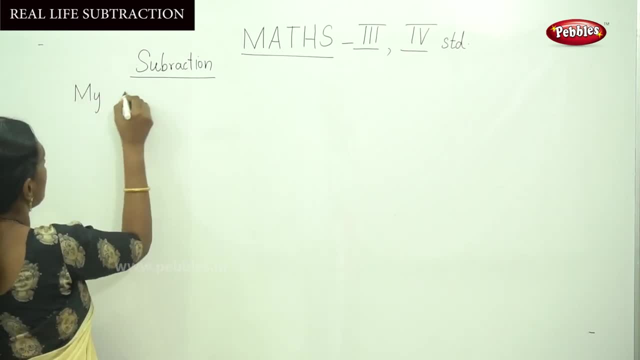 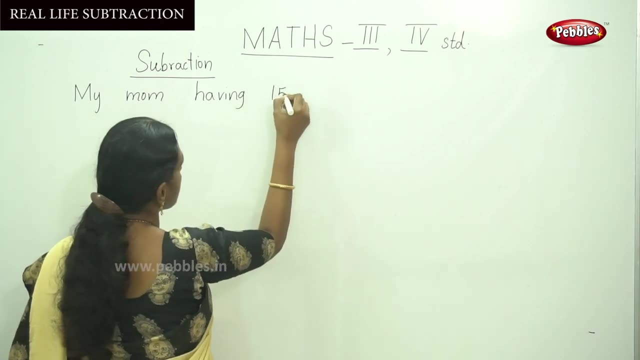 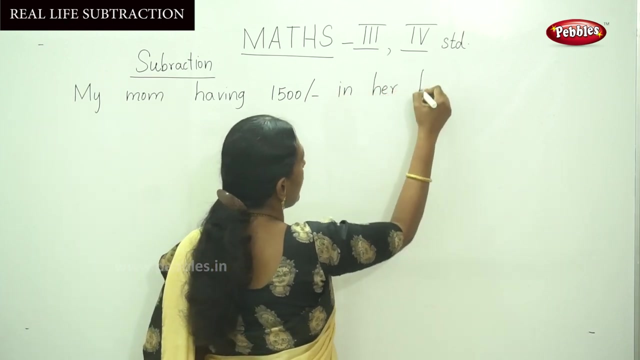 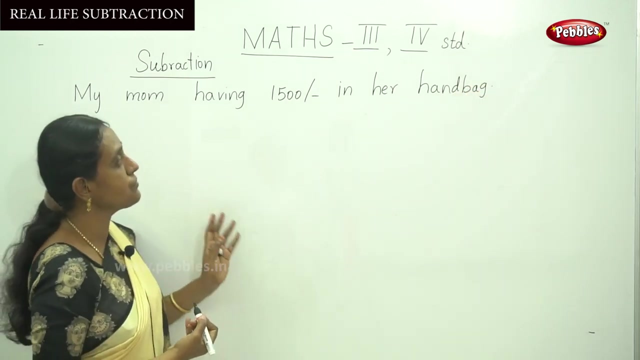 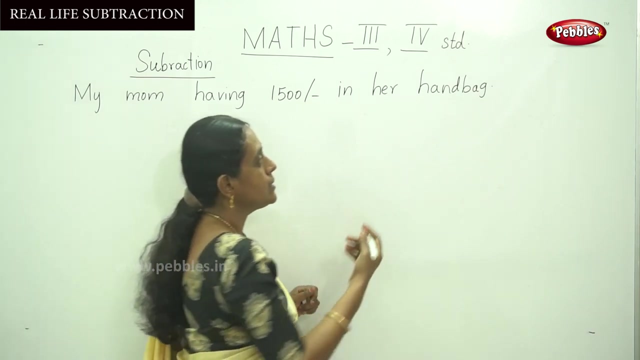 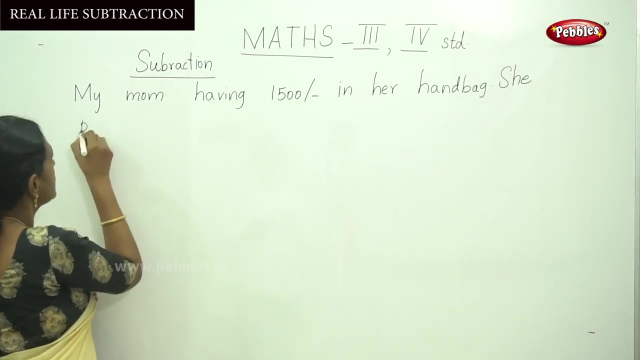 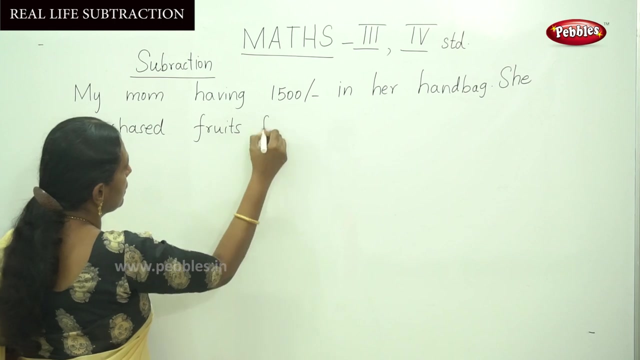 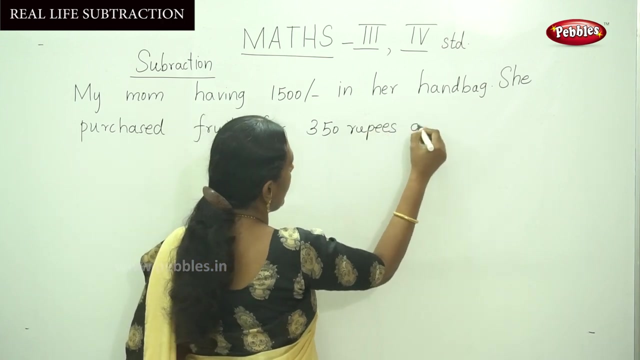 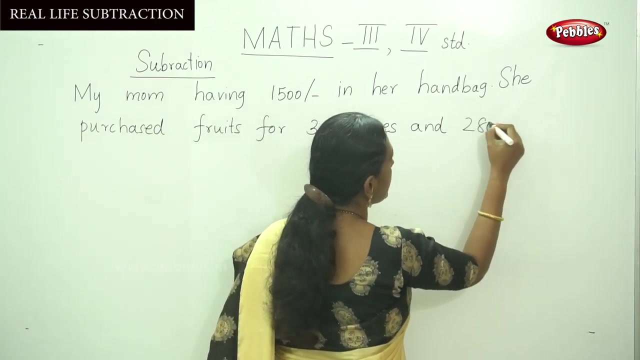 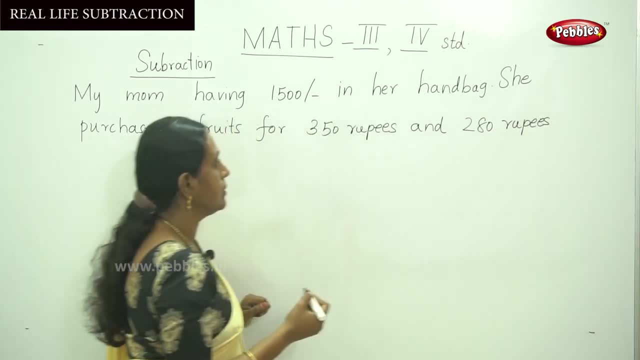 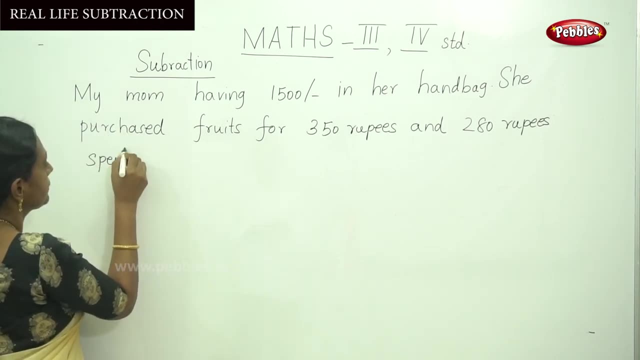 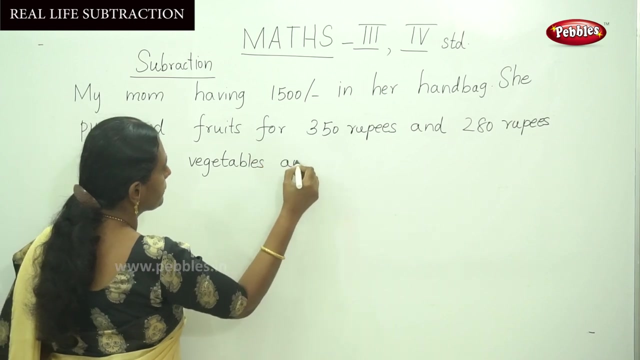 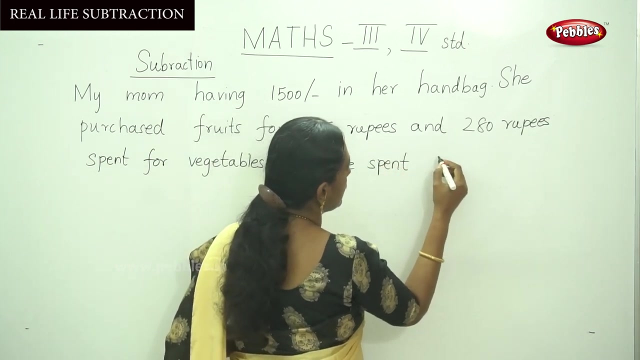 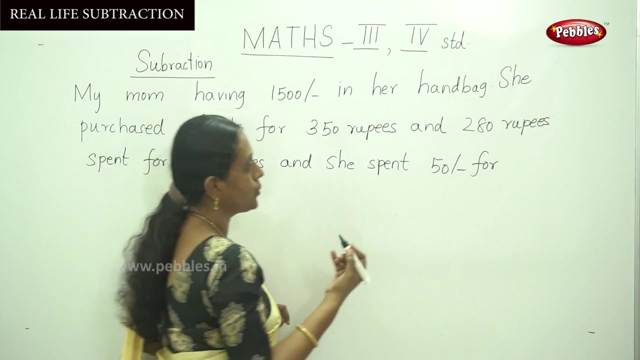 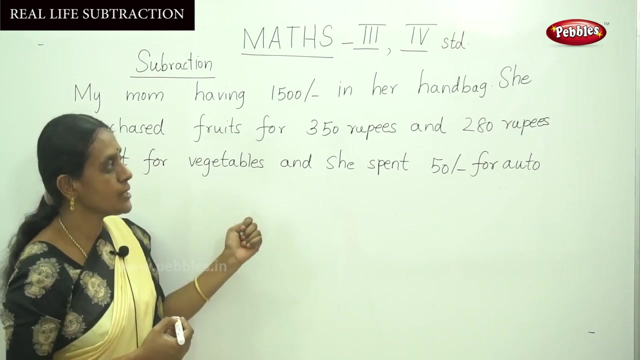 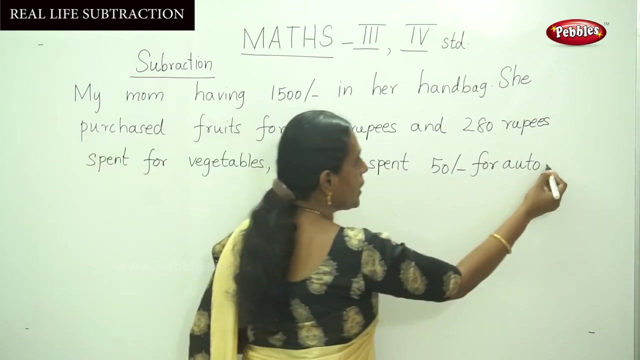 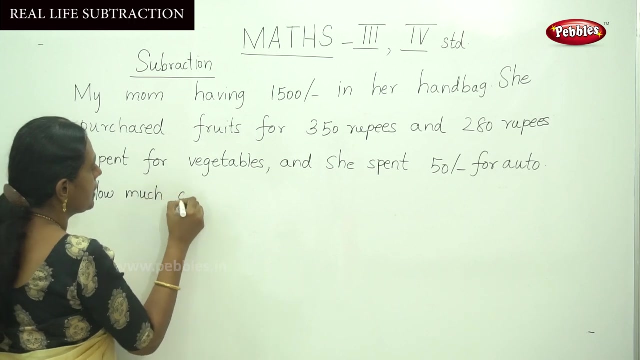 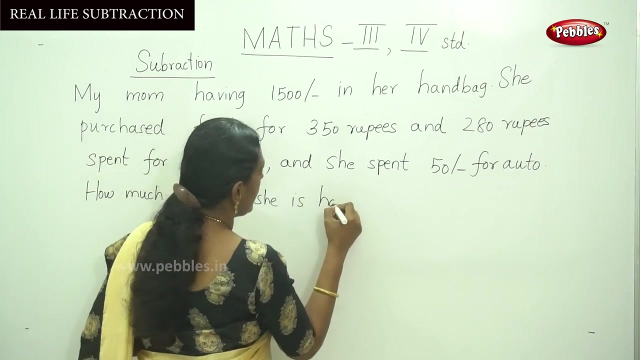 okay, she purchased fruits for 350 rupees and 280 rupees spent for vegetables. okay, and she spent 50 rupees for transport. okay, okay, for auto, anything. okay, purchased fruits for 350 rupees and 280 rupees spent for vegetables and she spent 50 rupees for auto. okay, how much the remaining she is having? okay, how much amount she is having. 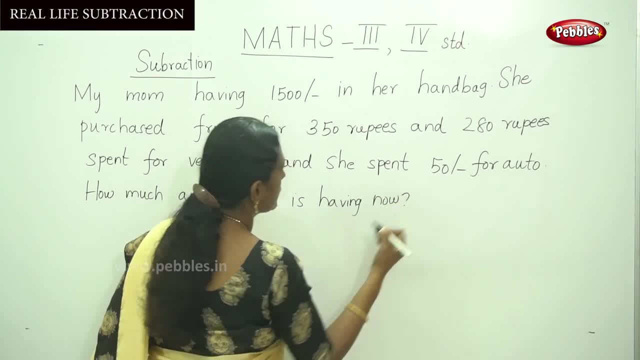 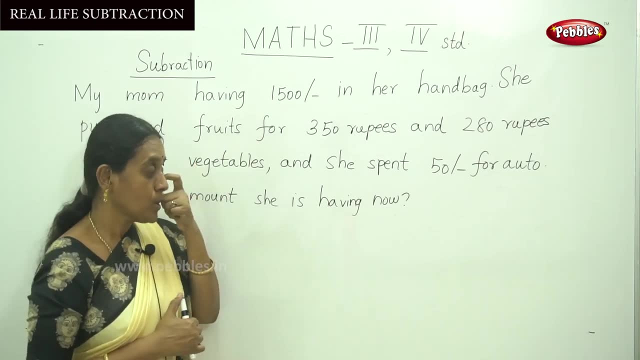 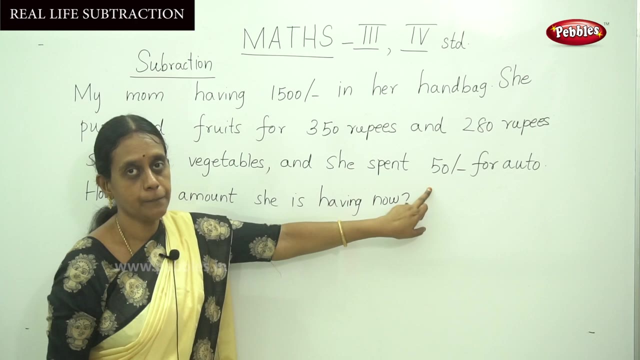 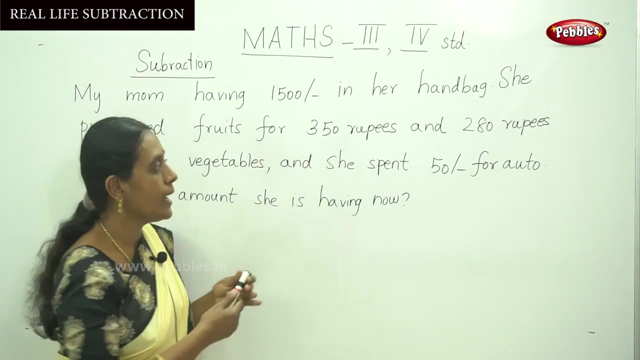 now, okay, so this is a real life situation. sum, okay, total amount is 1500, so you have to add this number, that is, 350, 280 and 50, because that is the spent money for fruits is 350 and vegetables that is 280 rupees and 54 auto. so you have to add these 3,. 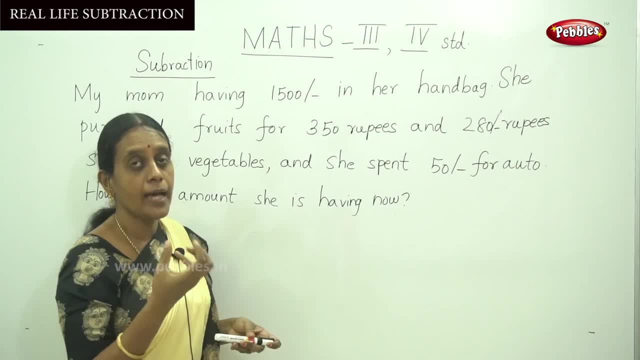 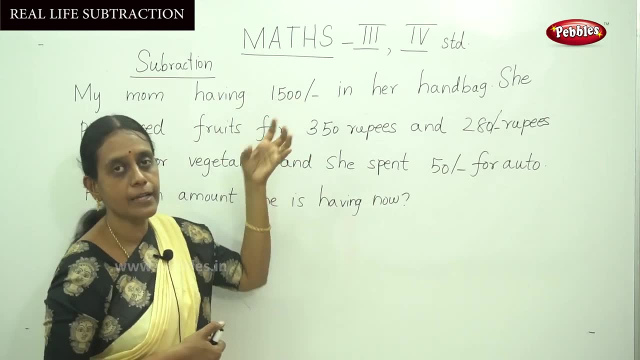 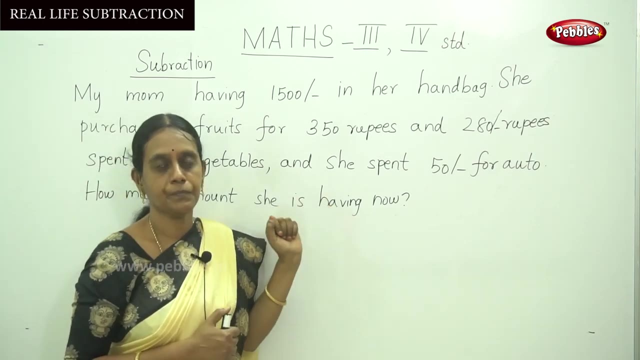 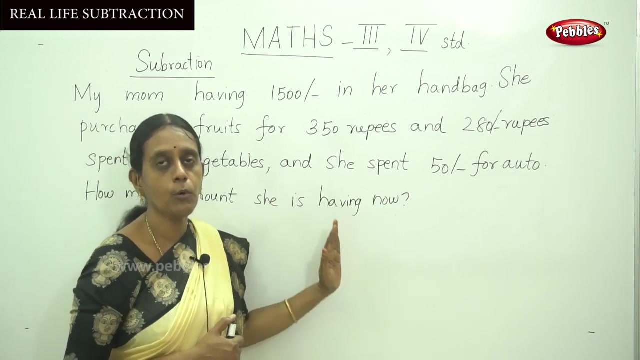 numbers. ok, find out the total number and you have to subtract that total sum from this total amount, 1500. so find out the remaining difference amount. that amount is she is having at last. ok, can you understand this? so you have to write down the step word problem. so you have. it is a statement problem. 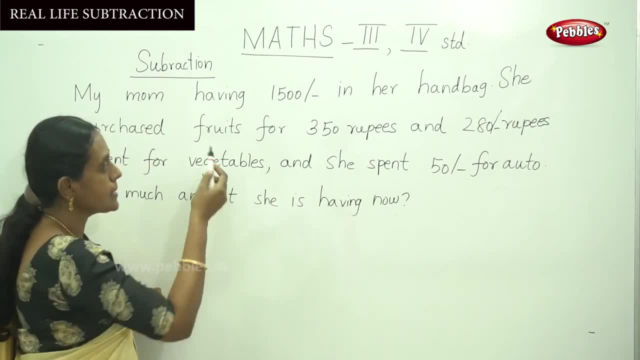 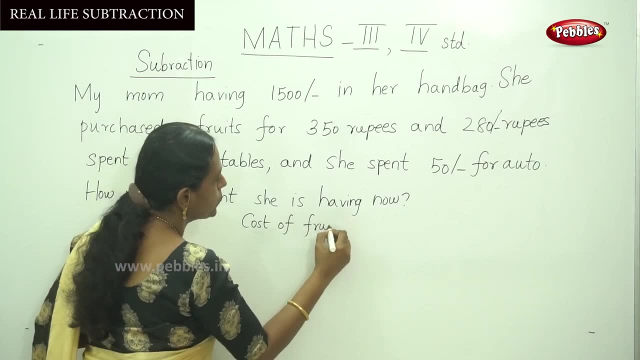 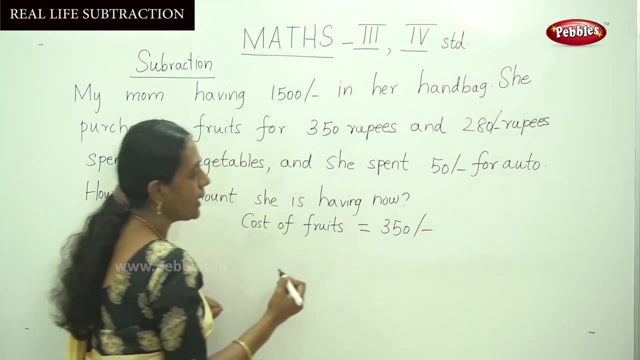 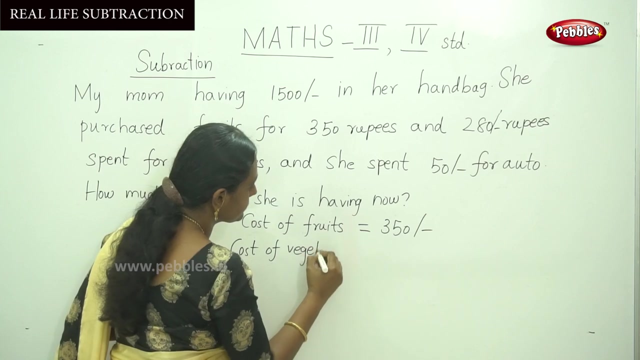 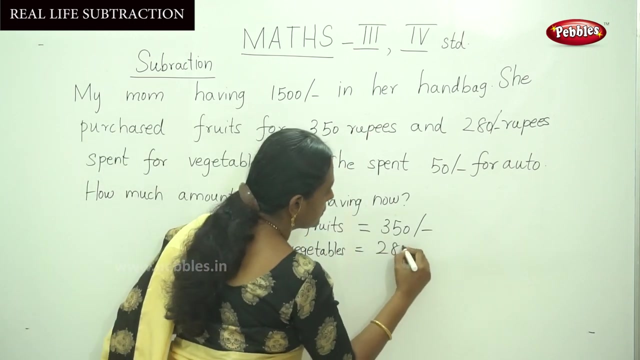 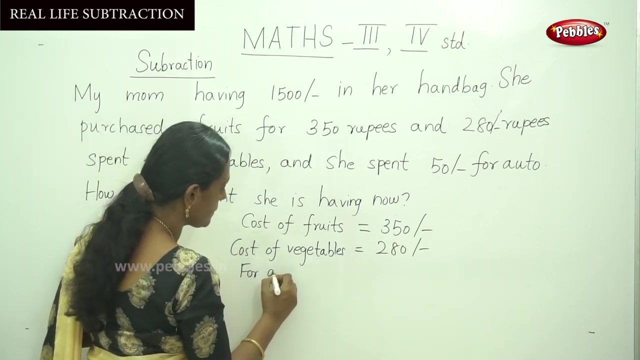 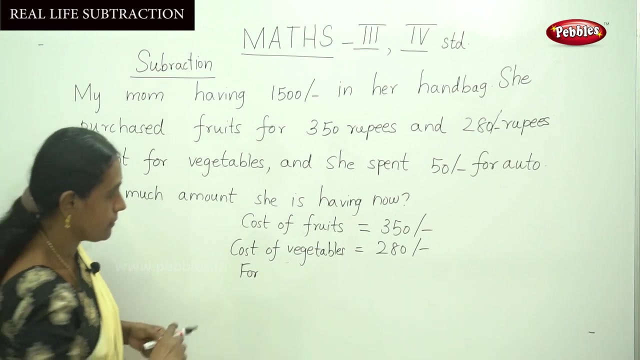 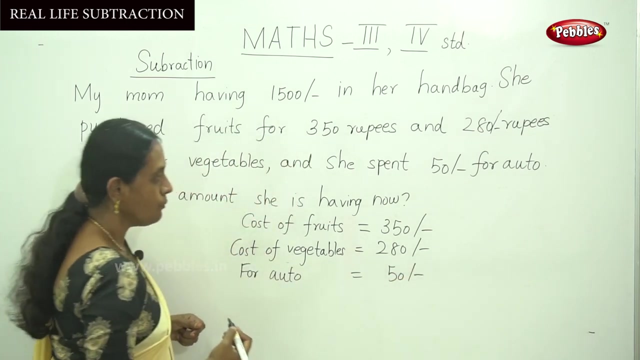 so you have to write down the question. ok, so that is cost of fruits, ok, cost of fruits that is rupees 350. ok, and that is for vegetables. cost of vegetables, that is 280, ok, and next that is transport for auto. she spent that is 50 rupees for rupees paise calculation. you have to write down this like because of that is. 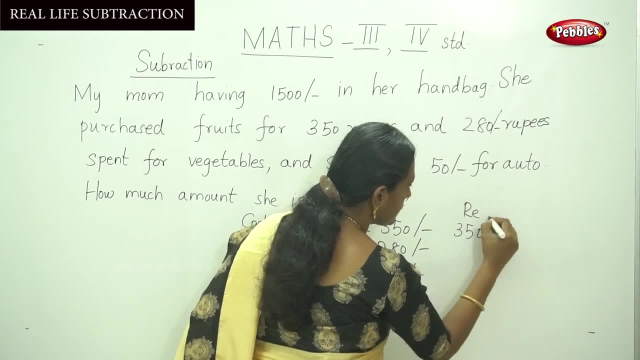 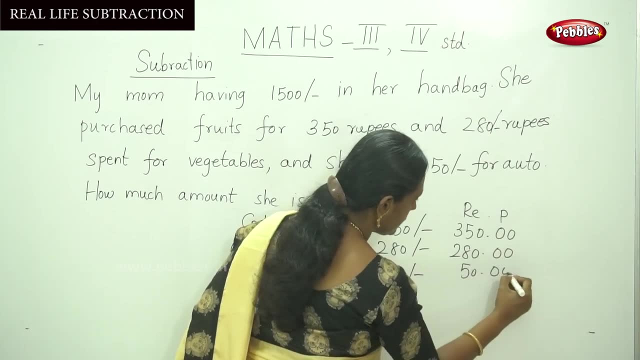 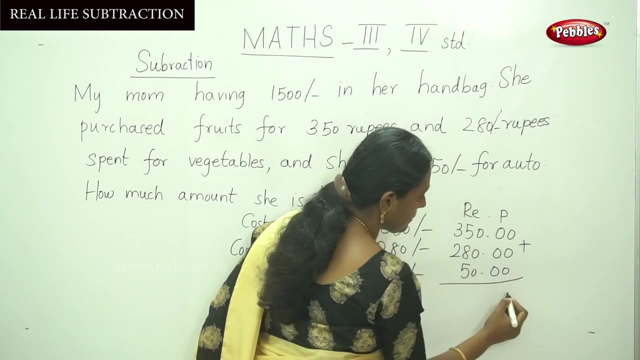 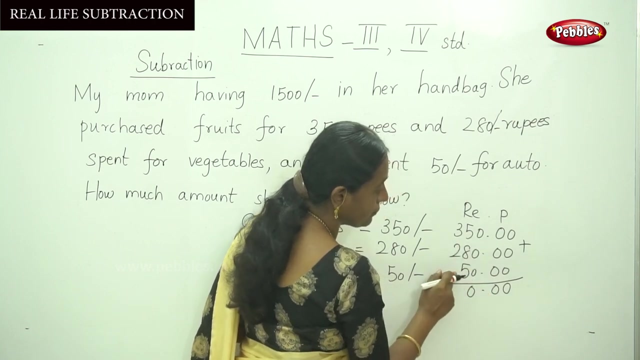 rupees paise. this is rupees and paise. okay, 350, 280 and 50, according to the correct place. that is column order, and first you have to add this number, that is 00. this is for rupees paise calculation. so 0 and 5, 5, 5 plus 5. 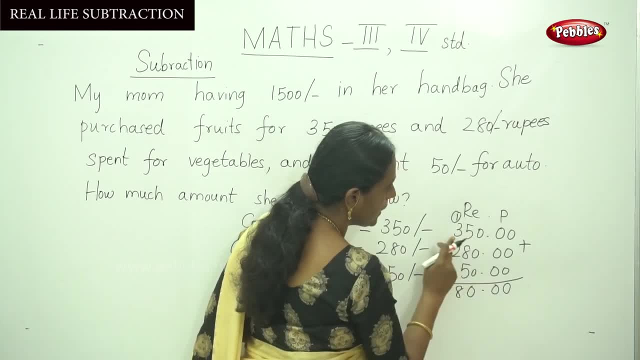 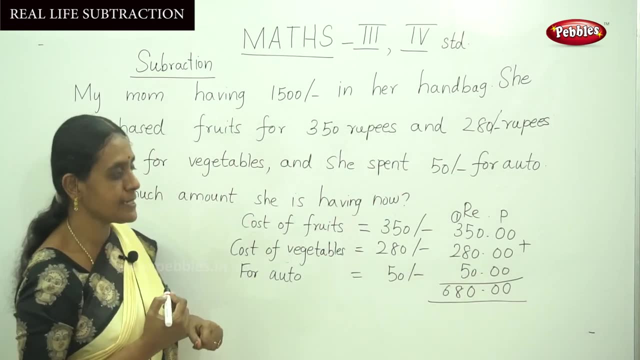 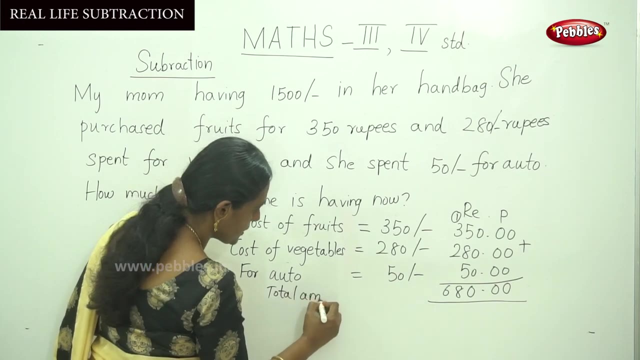 10, 10 plus 8, 80 and carry over this, 1, 3 plus 2, 5, 5 plus 1, 6. okay, the total amount she spent is 680. okay, this is a amount she spent, total. total amount she spent, that is 680 rupees. so the final question: 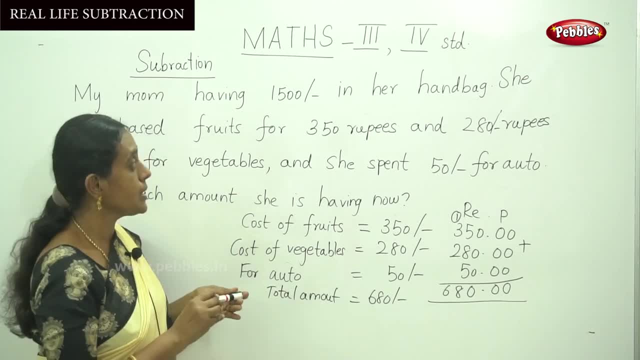 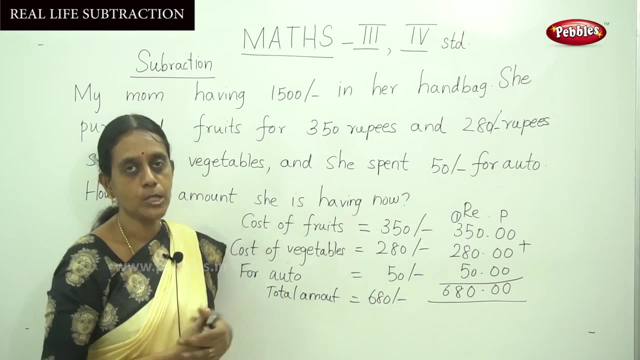 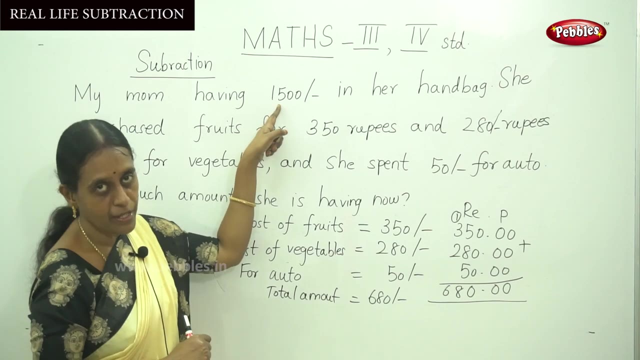 is the how much amount she is having now? okay, he is having first, that is, a thousand five hundred in her handbag and she spent 680 for purchase and transport. so how many, how much money is she having now? so you have to subtract the number. that is thousand five hundred, this 680. 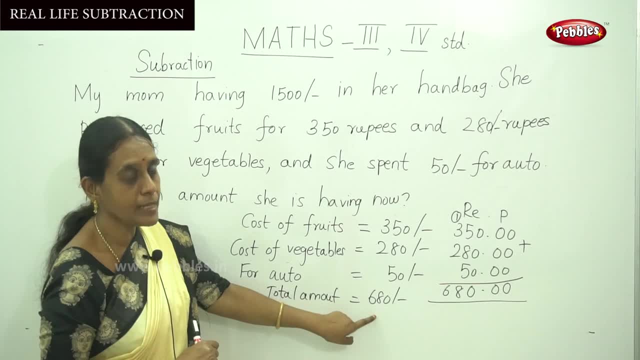 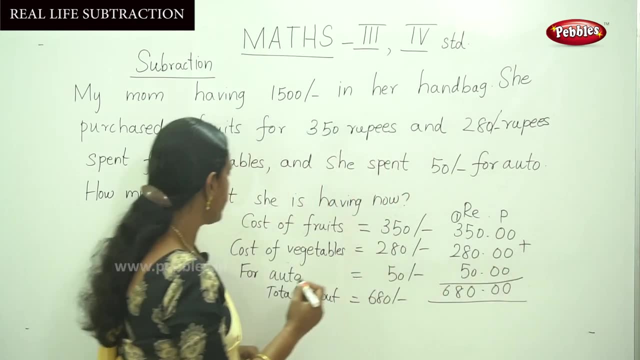 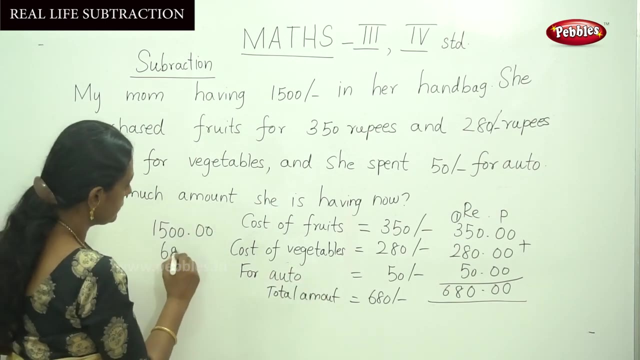 you can. this is sabrahan this 680. you can subtract the 680 from the minivan. okay, that is the final answer. so you have to subtract the number i'm doing here, that is, thousand five hundred, okay, and 680 minus okay, zero, zero. that is zero here. that is, you can't subtract the eight from zero. so 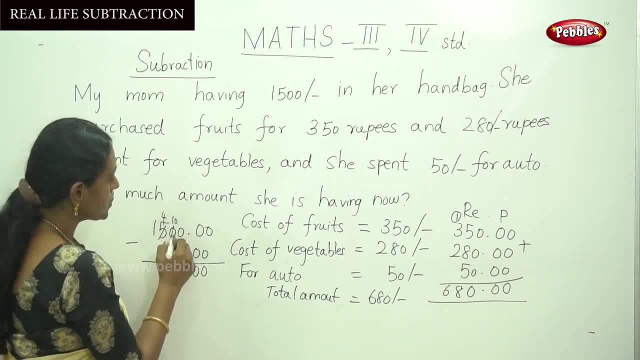 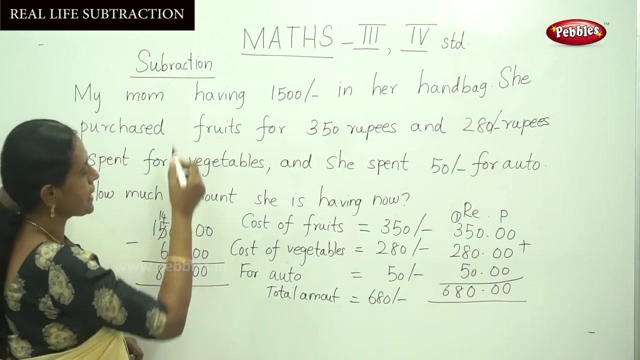 regrouping, that is, this is four and this is ten, so that is two, and again, you can't subtract the six from four. so regrouping, that is fourteen, that is fourteen minus six. okay, that is eight. okay, so this is a answer. that is remaining amount she is having is rupees 820. okay, that is the final.